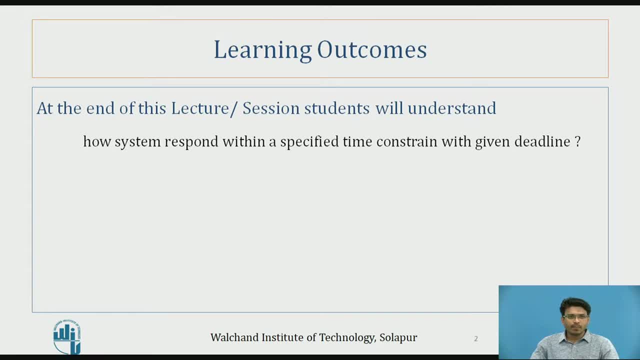 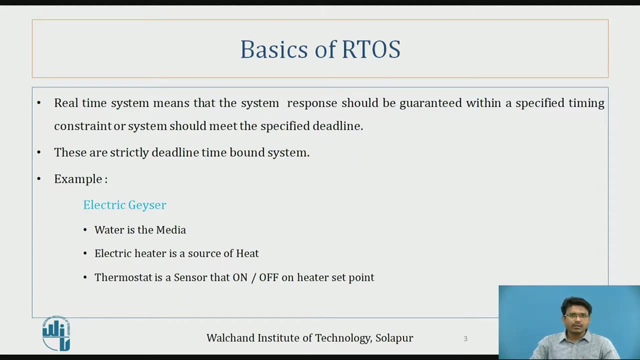 lecture or session, students will understand how system responds within a specified time constraint, with a given deadline. Let's start for the basics of RTOS. A real-time system means that the system response should be guaranteed within a specified timing constraint or system should meet the specified deadline in a given time. 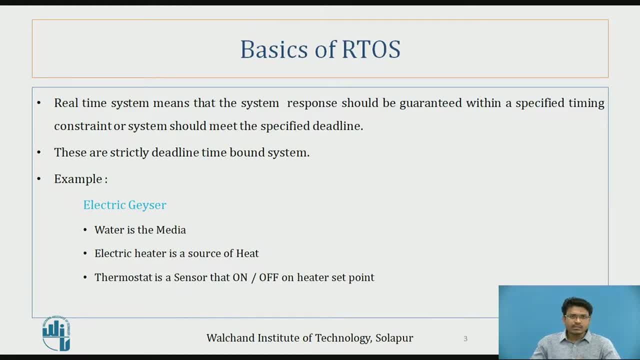 So now, what is RTOS? What we can call it is here. These are the strictly deadline. time-bound system Means. this type of operating system has made up for the specific task. They will perform the specific specified task within a specific time. It's like a chronological order, Like. 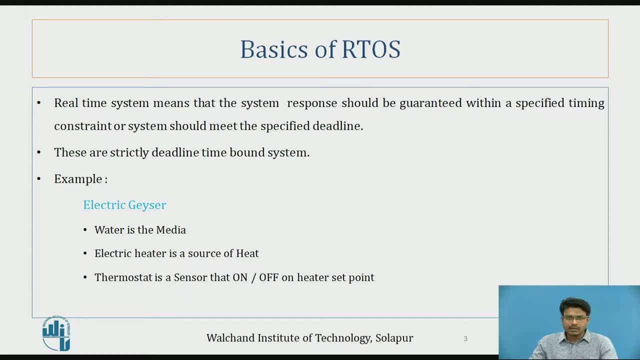 after completion of one task, it will go for the second task, then it will go for the third task. In this way, this RTOS system will work. Now let's we'll take the example of this RTOS Electric geyser. this electric geyser is nothing but the real-life example of RTOS. 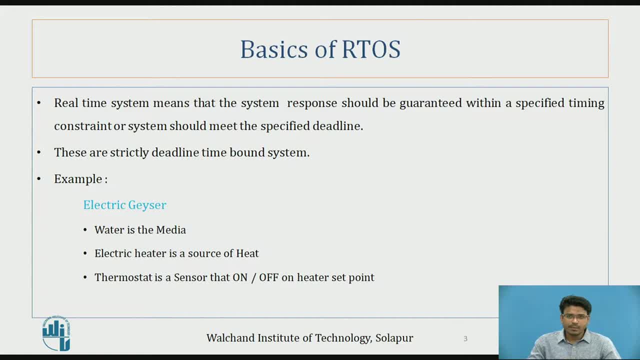 Now, in this electric geyser, water is the medium. Electric heater is a source of heat and thermostat is a sensor that on or off the heater's set point Means. in this electric geyser, to heat the water, we need to use a thermostat. Then what we do is: we have 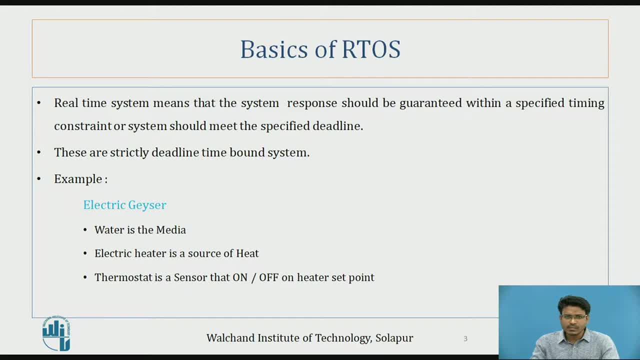 an electric geyser. This electric geyser is the source of heat and thermostat is the sensor- stat sensor. the role of this thermostat sensor is to check whether the water is heat or not. that is nothing but the electric geyser work. so now to perform this task. rtos will use means for. 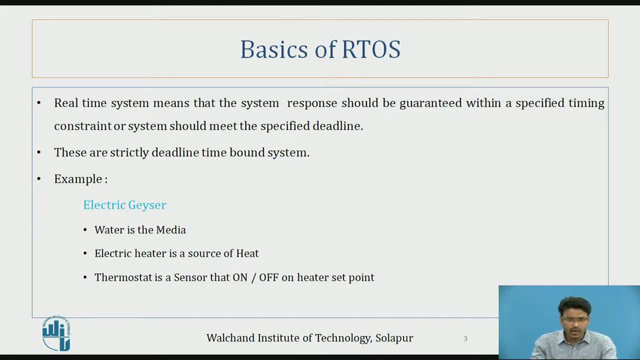 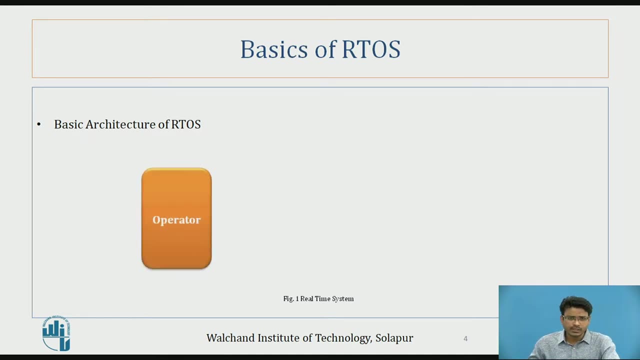 the specific time it will start the heater and after a specified time or set point it will switch off the headers. so now this one is nothing but the rtos, now basic architecture of rtos. now in this architecture, let's see, we have one operator and the real time computer system means 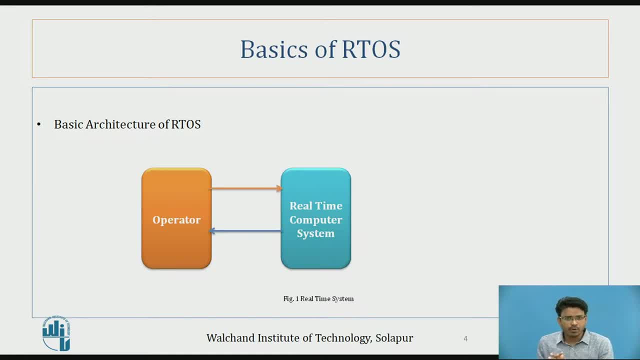 here the operator interact with the real-time computer system, and this is nothing but the man-machine interface means what in previous example: ellipse user will come into the bathroom and he will just switch on the geyser. so that is nothing but the operator and real time computer systems, man-made machine interface. but now, after that, 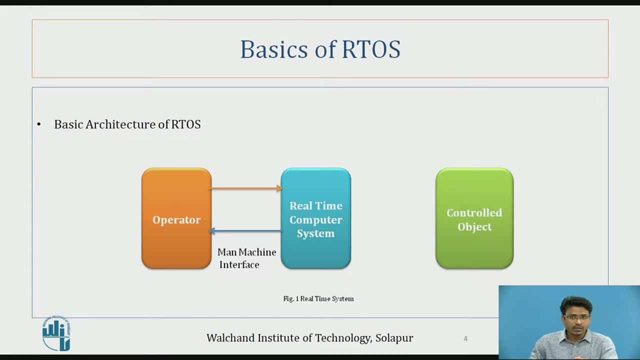 what happen? this real machine, real time computer system is going to interact with the controlled object. now, here controlled objects are nothing but the instrument. interface means here, like the thermostat sensor, that is the object, control object of this real-time computer system. so now, in this way real-time operating systems are going to be work. so now let's see the different types of 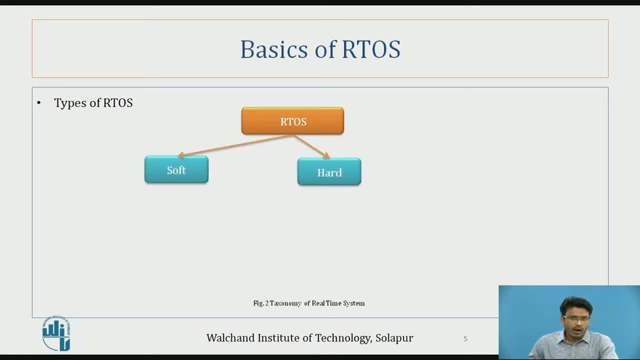 operating systems under this RTOS will have this soft RTOS and hard RTOS. now hard has again classified into the two things, that is the soft RTOS and the hard RTOS and the hard RTOS and the static and dynamic. and then dynamic is primitive, dynamic and non-primitive, and again static again. 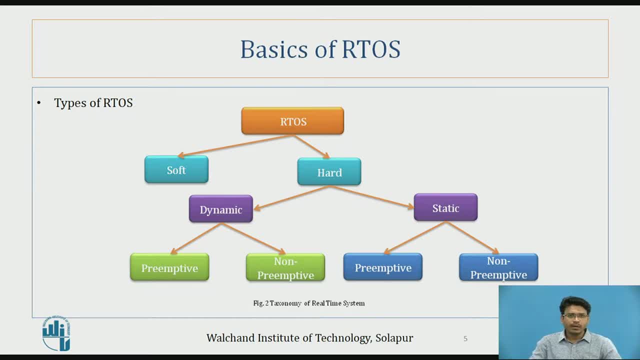 will have the primitive and non-primitive means. what here? in this type of RTOS, hard RTOS- the deadline is a fixed. it means anyhow, that system has to achieve the given task within a specified amount of time. that is nothing but the hard system. so now here the static and dynamic. now 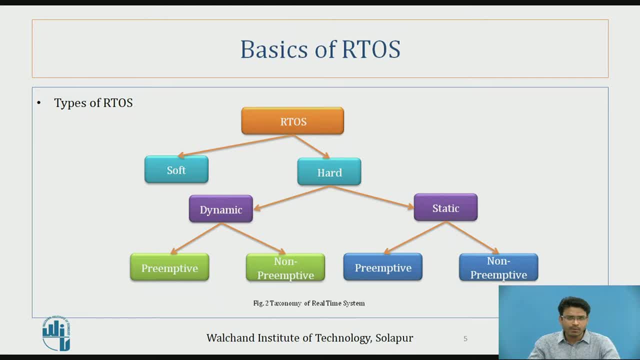 static means before going to start the execution of that program. it means before the compiler, at the time of compilation, we need to check. and now here, dynamic. it means while executing. if some of the tasks get wrong or something is wrong is happen, then dynamically, automatically it will. it will change the behavior and it will achieve the. 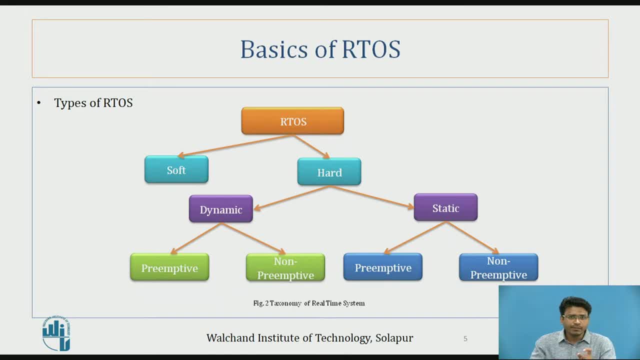 task anyhow. that is nothing but the dynamic. it means it will achieve at the runtime and a and in static it will achieve at the before runtime, that is compilation time. so now again here we'll have the primitive and non-primitive means. what primitive means? what it allows, the disturbance or 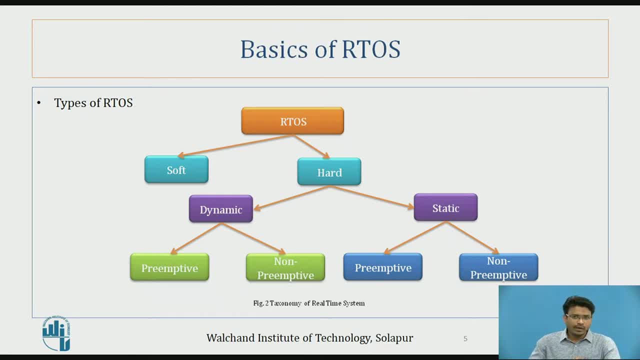 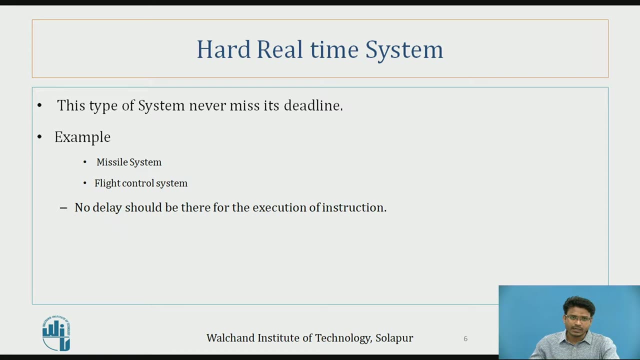 the interrupts, and non-primitive means it's not going to entertain any other process while executing its own task. so that is nothing but the non-primitive. now let's see the hard real-time system. this type of system never miss its deadlines, as already we have seen. so now let's see the hard, real-time system. this type of system never miss its deadlines, as already we have. 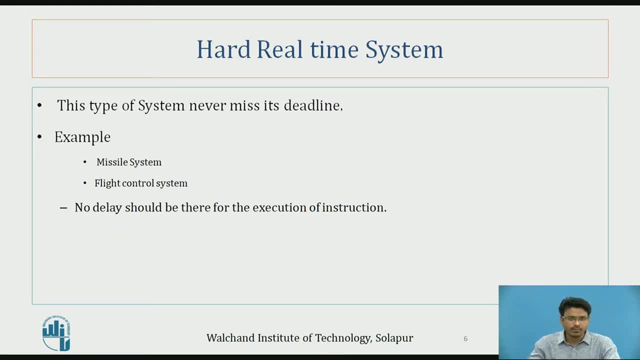 seen. so now let's see the hard real-time system. this type of system never miss its deadlines, as already we have seen. now let's take the example- is a missile system and the flight control system in the missile system. that is a missile engineering, right in in this system. there is no delay or no interrupt is allowed. that is. 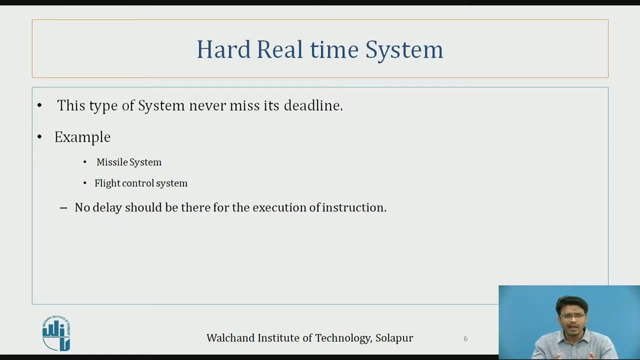 the missile system and even the flight control system, because there is the n number of flights in the air. so at that time, if something get wrong, then maybe there will be the chances of flights to get a collide. hmm, so that is nothing. but the hard real time system means there is no delay allowed in this system. now, soft in the soft real. 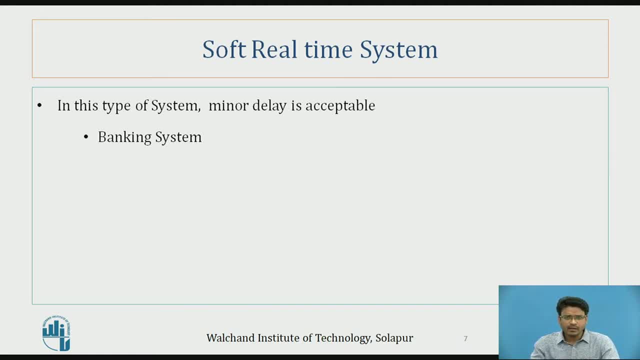 time system, it will allow for the minor delay. it means like take the example of banking system in banking system, getting the cash withdrawn in the hand. maybe it will delay no second or two seconds, it doesn't matters- while transferring the amount from one account to the another account. 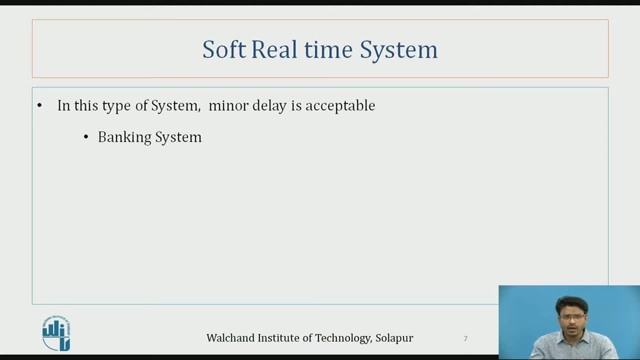 it will take some time. actually, it will always vary the time between these transactions. so that is the very minor delays acceptable in the soft real time system, so that one is nothing but the banking. now let's talk about the terms related to the rtos. now, first term is job. a job is a small 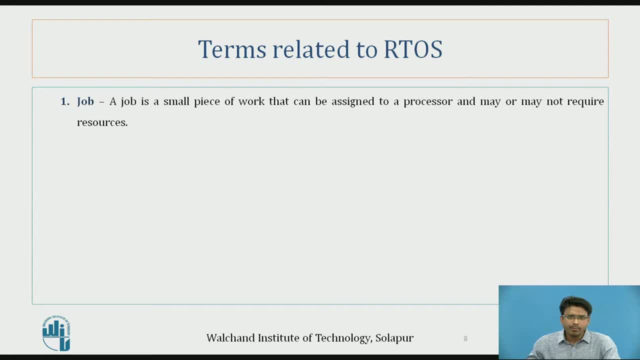 piece of work that can be assigned to a processor and may or may not require the resources. that is nothing but the job and task. a task is a set of related jobs that jointly provide some system functionality. next one is a release time of the of a job. it's the. time at which job becomes ready for the execution. that is nothing but the real time of a job. execution time of a job means it is a time taken by a job to finish its execution deadline of a job. it is the time by which a job should finish its execution. 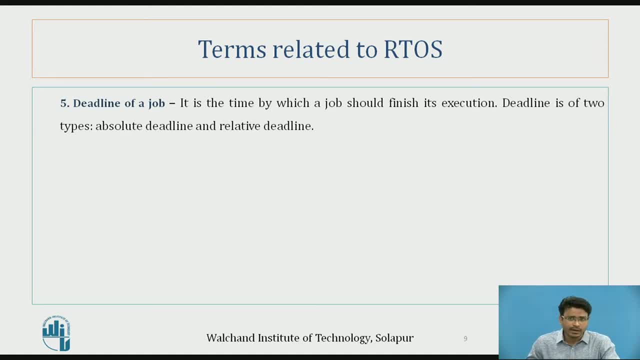 deadline is of the two types again: absolute deadline and relative. we'll see in the next slides. so now here the relative deadline. the maximum allowable response time of a job is called the relative and in absolute deadline of a job is a equal to its relative deadline plus its release time. response time of a job: it's the length of time from release. 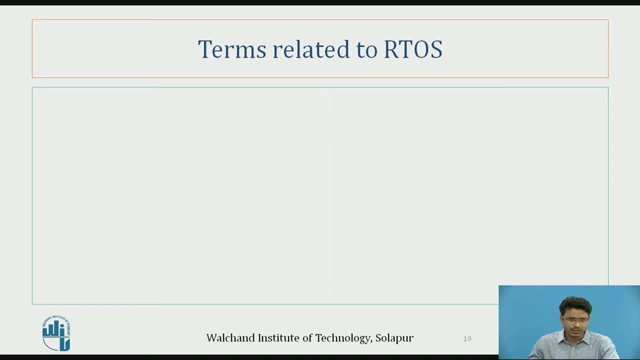 time of a job to instant when it finishes. now, processor are also known as active resources in the RTOS. they are essential for the execution of a job. a job must have one or more processor in order to execute and proceed toward the completion. my examples are the computer systems. 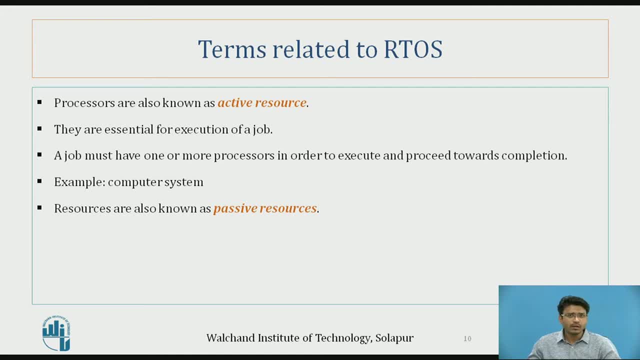 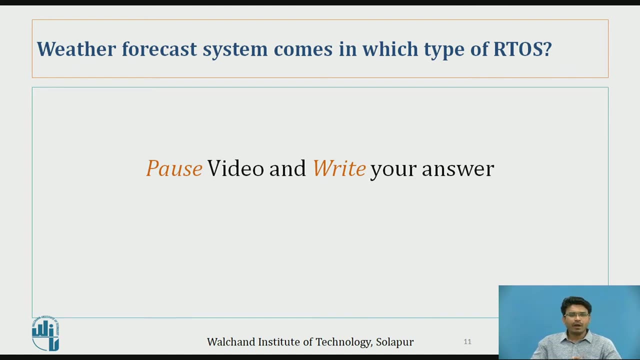 resources are also known as a passive resources. a job may or may not require a resource during its execution, for example the memory or mutex. now, here let's see one question. now we have learned, like, what is mean by hard real-time system and soft real-time system, and all now here, just tell me whether forecast system comes. 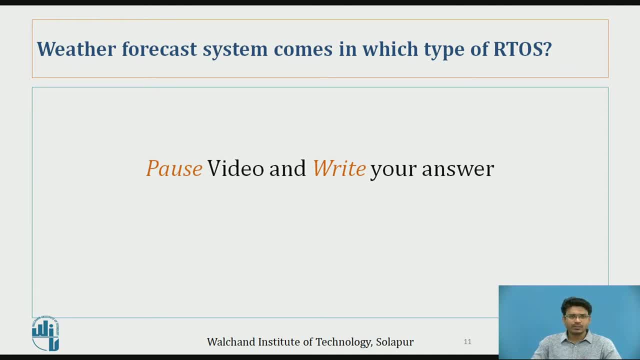 in which type of RTOS? pause the video and write your answer. now here it's. the answer is by using soft real-time system, because in a weather forecast system there will be some delay, will be acceptable means while I am getting the weather of my current location wherever I am, I will get a some different results many times because if I will check for the 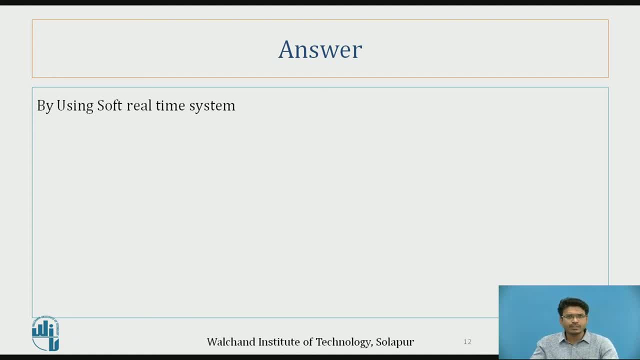 in the morning, 10 am, I am getting some results, and after I will check the ten point five am. now again i am getting some different results. so that is nothing, but some delay can be acceptable. that is nothing but the soft real-time system. now let's see one case study: the real-time. 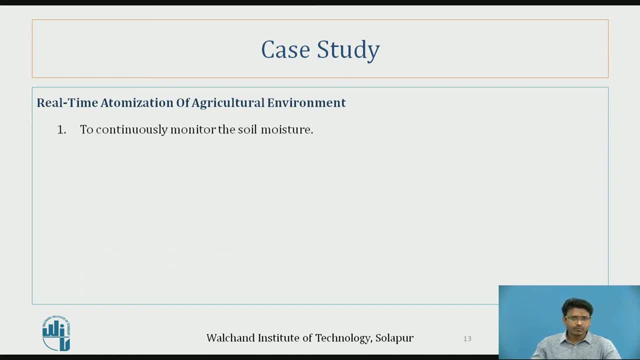 optimization of agriculture environment. to perform this agriculture environment for the real-time system, we need to consider some parameters like to continuously monitor the soil moisture. this can be done by some sensors. then we need to continuously monitor the water level of the well. then again, we need to check the temperature, humidity and dew points. so as far forecast.